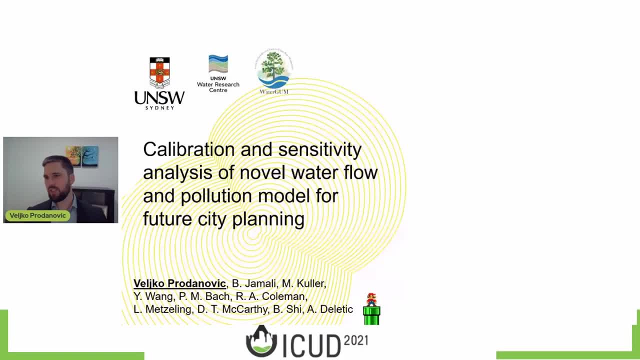 Hi, Thanks, Tone, for the great introduction, Everything true, And great pronunciation of my name. by the way, I'm also very honored and humbled to present today at the Paul Haramos session, and alongside the other two incredible finalists. So let's jump straight into it, right. 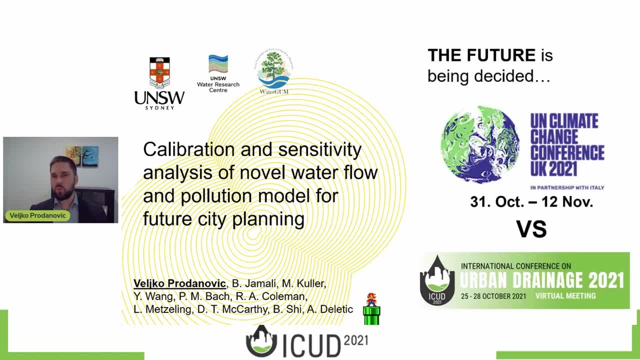 So when we talk about the future, there are two ways we can plan for the future. One way is by attending the climate change conference that is actually happening next week and sitting in a room full of people that we might not trust and talk about things that won't actually happen and we won't actually do them. 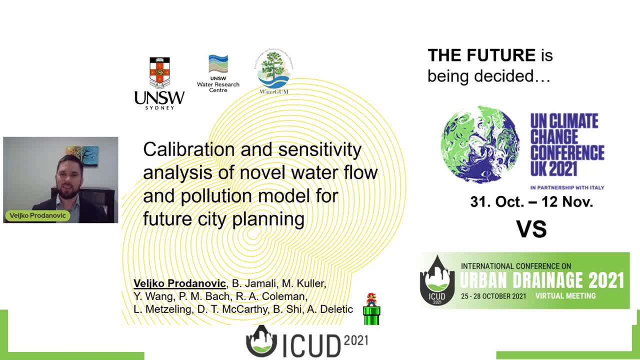 Or we can attend ICUD and discuss our amazing future of urban drainage with our respectable colleagues. And I mean, guess what? I'm here And I think this is a much better choice to do it, Do it. And so let me introduce you my idea today about exploring the future of stormwater pollution by using the future urban stormwater simulation model, or FAST model. 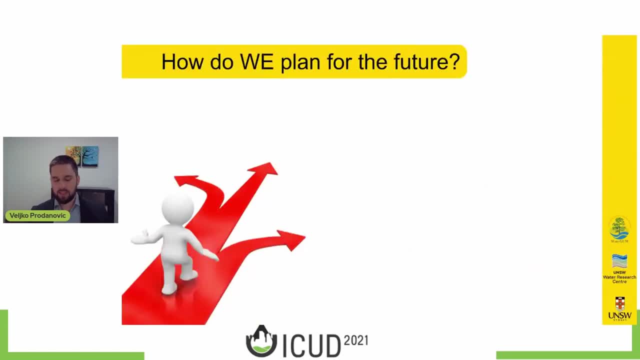 So let's jump into it, And I'm going to start with a question, hypothetical question- But do we, as urban water engineers- As many of us as we have here today- Actually know what cities are going to look like in 10,, 20,, 50 years time? 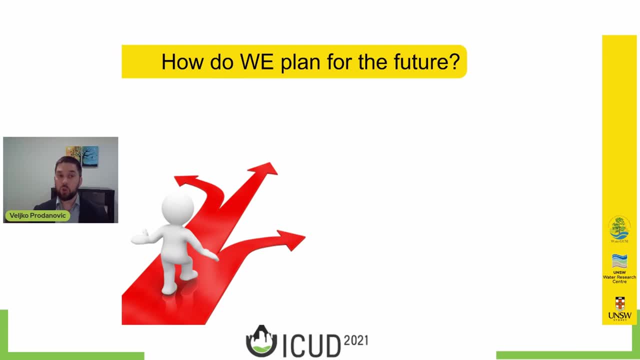 We don't right. We have no idea what it's going to look like, but we do want to know, because knowing exactly how much flows we have and how much pollution we have in the catchment Amazing like easy life right, Because we can plan better. 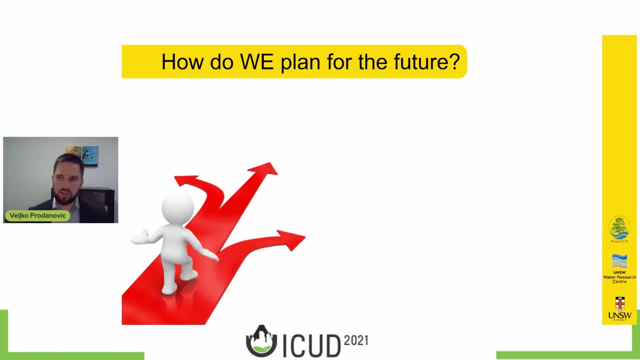 But today, in 2021. Is there actually a good way of predicting what our cities are going to look like in the future? Well, I mean, of course, not actually, And I'm sorry if you're expecting me to present today some revolutionary piece of software that solves all of your problems and predicts exactly what future it is. 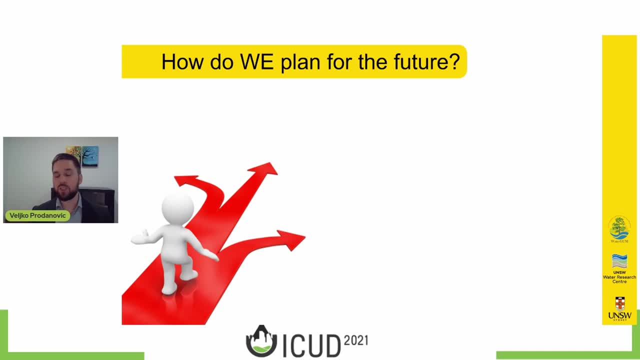 Just doesn't exist, that that kind of technology doesn't exist unless you have a time machine. So humans are so very unpredictable And we don't know what's going to happen in the next hour. We don't know what's going to happen, what the priorities are going to be over the next course of period. 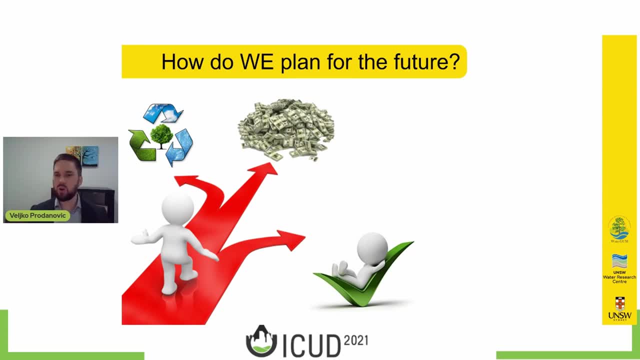 Is it going to shift in an environmentally positive way, or are we going to chase money as we usually do, Or is there going to be some other political agenda that will shape our cities? The future is so uncertain, So, but still, that does not and should not mean that we should. 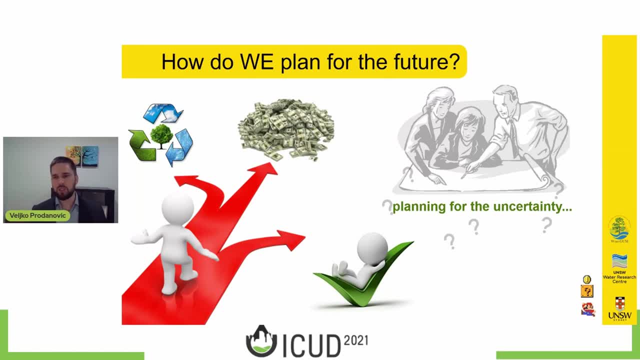 So uncertain, But still that does not and should not mean that we should. We should start planning for different uncertainties and different futures. We should start exploring what those futures might look like And our development of our cities depend on that development of our climate and how climate affects our planning. 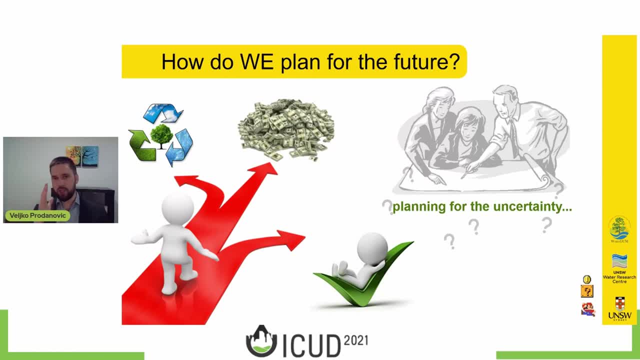 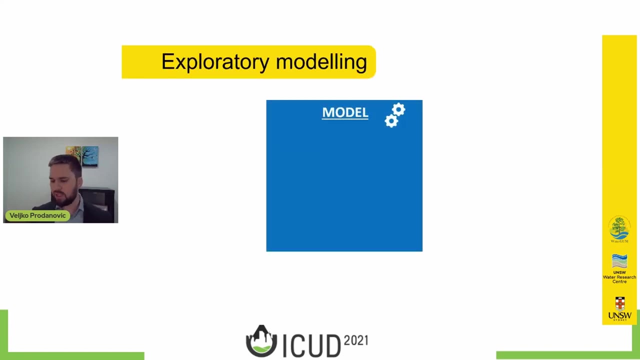 All that is intertwined, But we should not try to predict one future because there's no. there's no one future. There is a multitude of possible futures, So we should explore Rather than predict. So, when talking about exploratory modeling, what are some of the key parts of the exploratory models that we should consider? 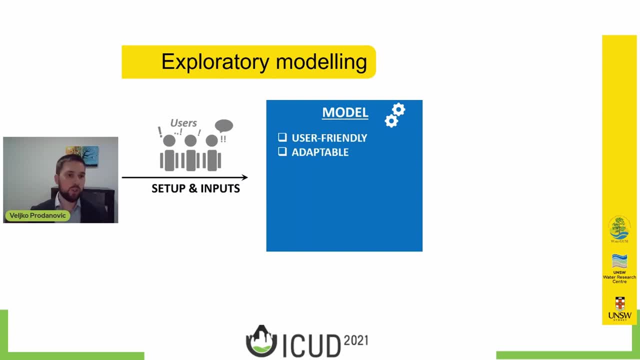 Firstly, we have the users And as a water engineer, I tell you now we don't have a luxury anymore just to talk to the scientific community. Our models should also cater to those guys that are meeting next week and we should try to give them a user friendliness of our model. 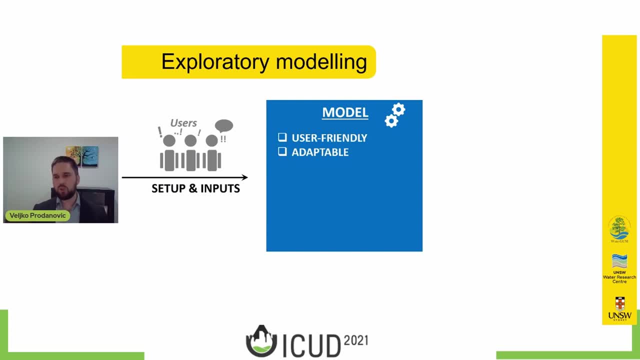 And the solutions that that we offer. So the models need to be adaptable to different desires and different stakeholders that want to engage with them. Also, we live in a fast paced world. There's instant gratification everywhere. You can get anything on demand. 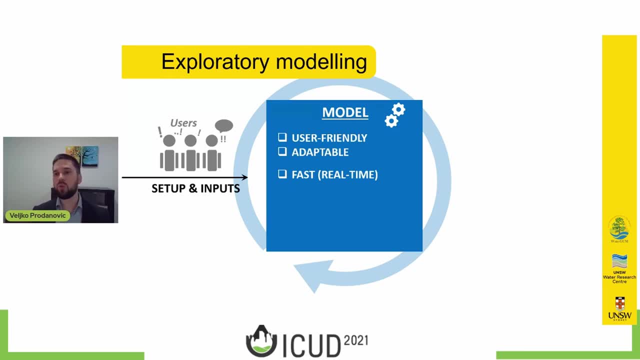 So our models also need to be the similar way. So they need to be fast, They need to work in real time And once we get some of the outputs again we need to cater the outputs to the actual users. So we 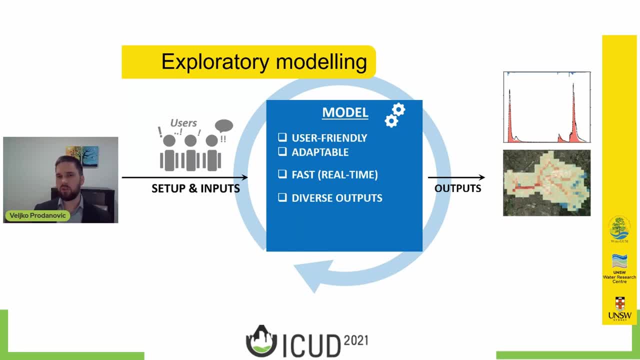 Can have more scientific outputs, but we also need to have more illustrative outputs which are easier to understand and present. Finally, once we get the outputs, it's inevitable that someone will say: this doesn't make sense. I don't like this. 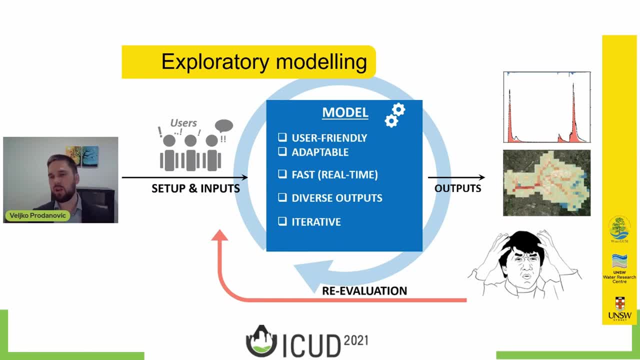 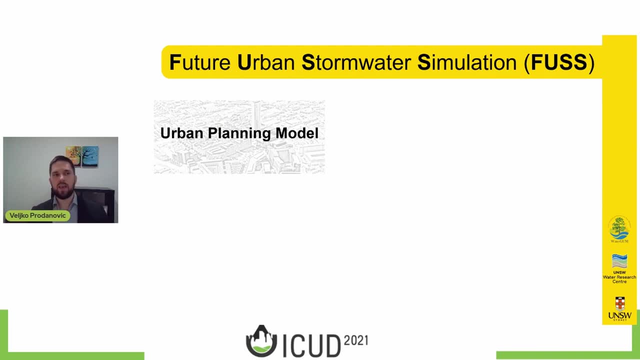 So the models need to be able to iterate through the possible scenarios. So when designing such exploratory models to understand the future of stormwater and stormwater pollution in our catchments, we first need to look where we live, So we first need to know how our cities are developing. 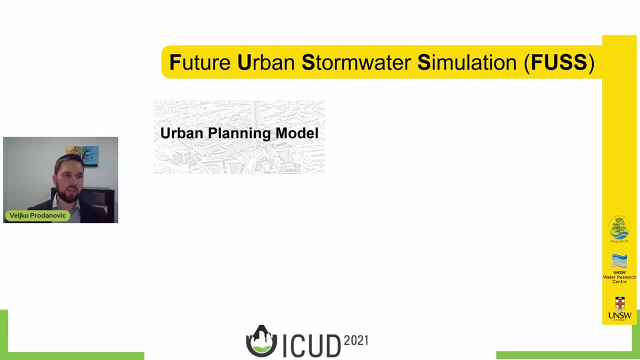 In order to know that we are using urban planning models, So that urban planning model needs to be the first step in determining what are some of the activities in the catchment, And my colleague previously talked about how impactful these activities can be to our stormwater pollution. 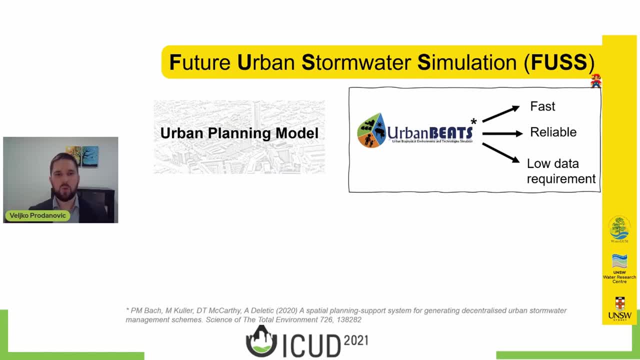 So for this particular work to our FAST methodology, we use urban planning model called UrbanBeads. UrbanBeads creates the abstraction of urban environment using urban planning rules, So it simplifies it and it's found to be fast, reliable and has quite a low data requirement, which is great for exploratory modeling. 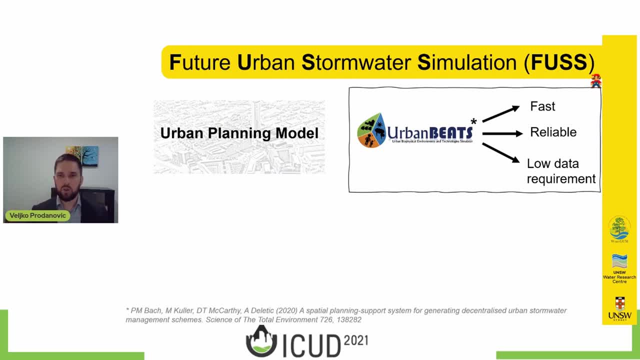 I'm not going to talk much about UrbanBeads today, but you can check out the publication below, And my colleague Dr Peter Bach is probably somewhere here on the chat, So Please catch up with him for more info on UrbanBeads. 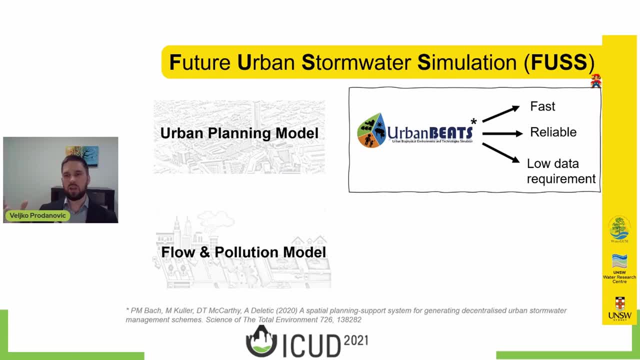 Next, once we know how a city is developing in the future, we attach a quality and quantity model to it. So there are pretty much similar requirements for that. So we need low data requirements again, because we never know how much data we will have for the future scenario. 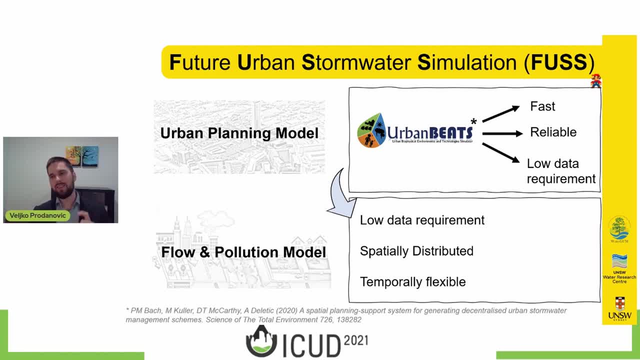 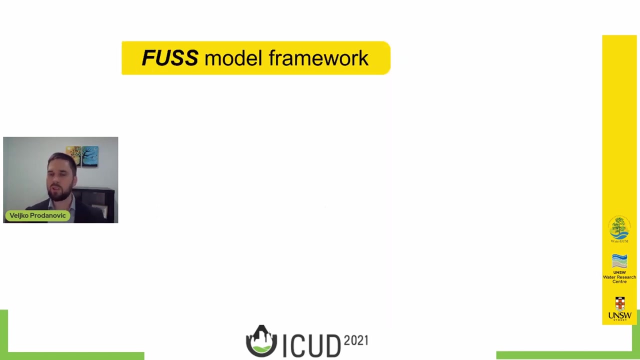 And the models need to be flexible in spatial and temporal Scales so we can interpret the different types of scenarios. So for our FAST methodology, we coupled UrbanBeads with the modified EPA SWIM methodology to achieve this. Okay, so let's see what all the FAST is about, right? What is the FAST? What does the FAST represent? 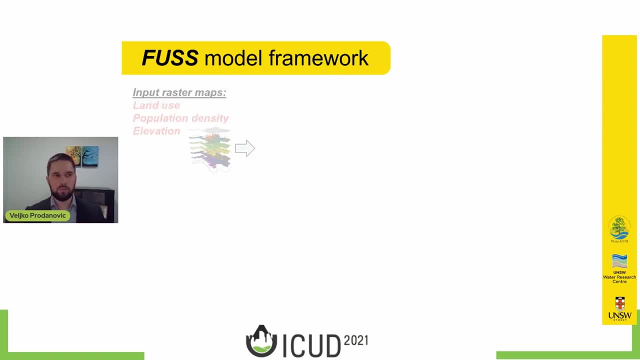 So this is the core of the FAST methodology. So we start off with a very simple input maps which are RASP and RASP2.. These are the maps readily available to almost any user online. We feed them to the UrbanBeads to create spatial representation and delineate dark catchment. 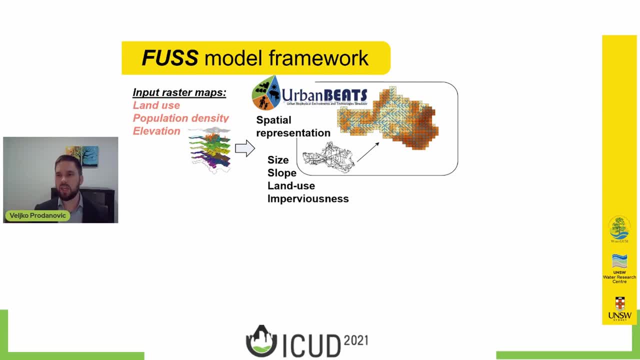 UrbanBeads creates these blocks, which are user-defined, which contain information on the size, slope, land use and imperviousness. So next we feed these blocks and transform them into SWIM subcatchments. There are two layers that we create in SWIM subcatchments. 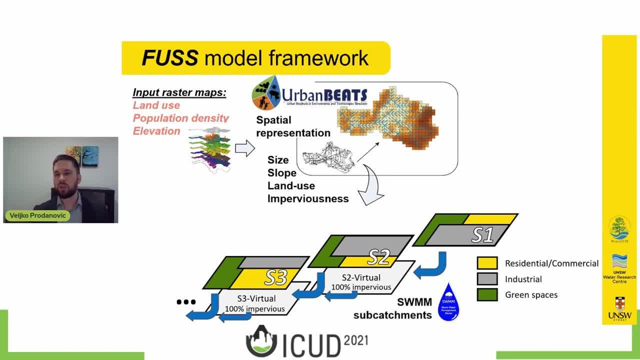 real subcatchment and the virtual subcatchment underneath. So the real subcatchment gains all the physical attributes from the block and in current model we consider three different land uses for it: residential, commercial, industrial and green spaces- and the proportion of these land uses is dependent on how the city is developed. 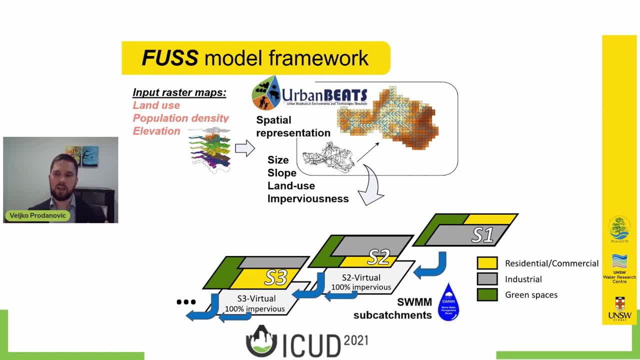 within urban deeds. The second layer of subcatchments are the virtual subcatchments which actually replace drainage pipes in our system. So it simplifies the model and requires less data, requires less simulation time. They have exactly the same physical attributes as their parent subcatchment but 100% impervious. 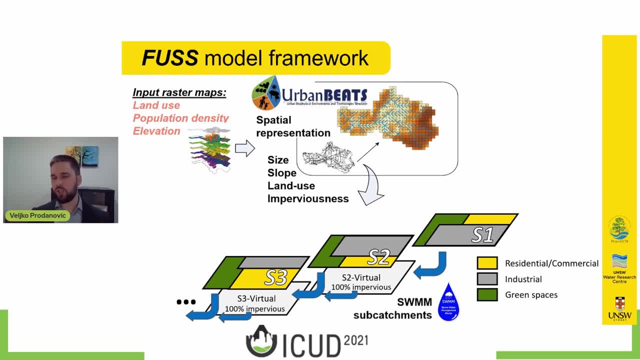 and act basically as a pipe, So they don't add additional flows of pollution. The only other input parameter that we add here is a continuous rainfall series. So it can be, if you're calibrating. So that's a current rainfall series. 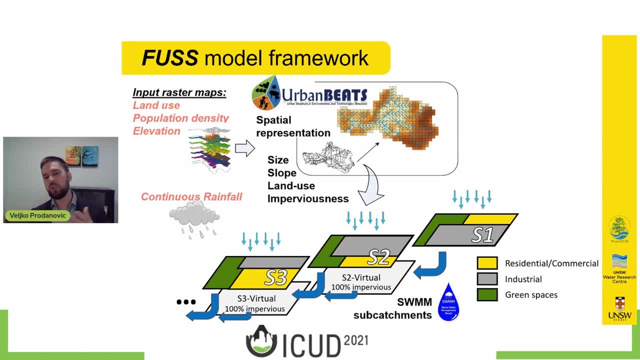 Or some of the years you're calibrating for, or if it's a future, it's a generated future rainfall series. We need rain for stormwater to work right. And this leaves me with the final aspect, and that's the human activity in the catchment. 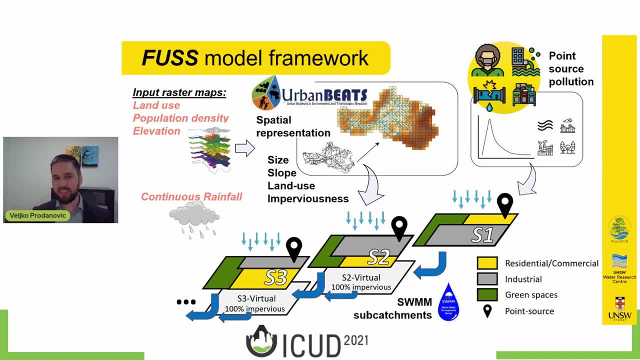 So again, we saw in the last presentation how important these things are. So what we did is added point source pollution to each of the subcatchments. These point sources are stochastically sampled From the data gathered and adding flows and pollution into the catchments. 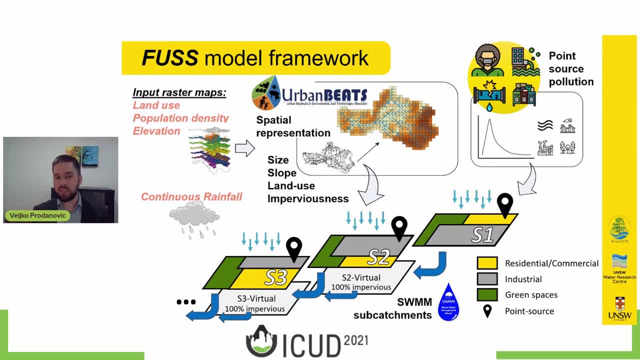 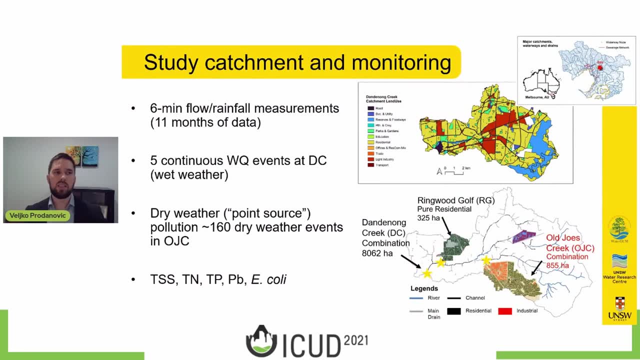 So the combinations of all these elements make the FOSS model and the FOSS methodology quite unique. The model was applied on Dandenong Creek catchment, which is approximately 8,000 hectares in size. It's in the Melbourne Victoria. 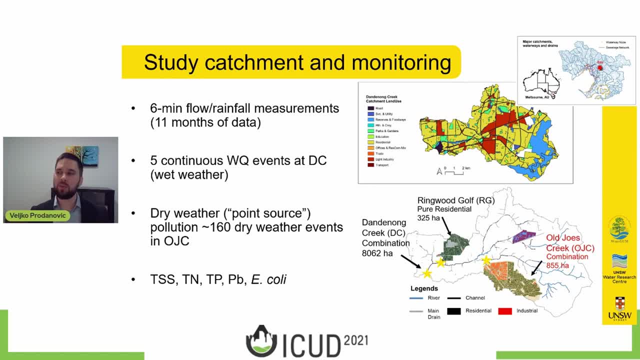 Australia And there are two other smaller subcatchments within that catchment called Ringwood Gulf, which is purely residential catchment, and Old Jaws Creek, which is a combination of industry and residential. There were 11 months of water quantity data and the rainfall data that we used with five. 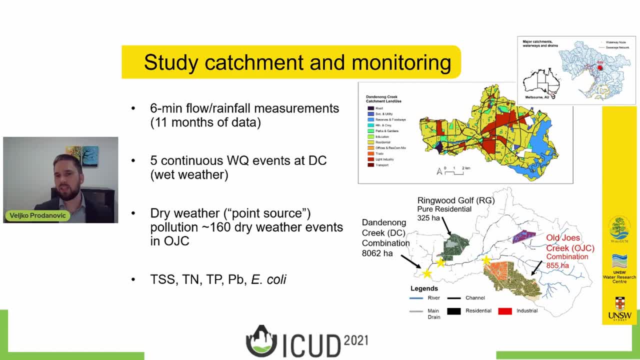 continuous water quality events and the dry weather, which was again, thanks to my previous colleague, gathered on the Old Jaws Creek site, used to generate these stochastic relationships of the dry weather flows. All the pollutants, all the sorry- all the samples have been measured for total suspended. 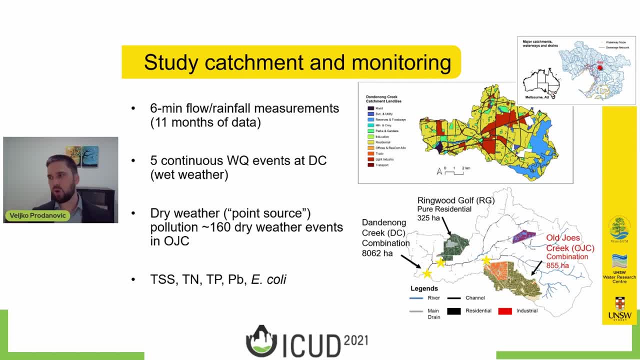 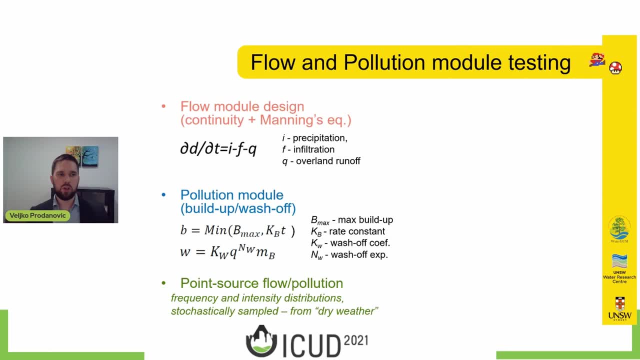 solids: nitrogen, phosphorus, lead and E coli. On the technical side, flow model of the FOSS methodology uses continuity and Manning's surface runoff equation. We The The linear buildup and exponential wash off. The point sources for flow and pollution again was stochastically generated from these. 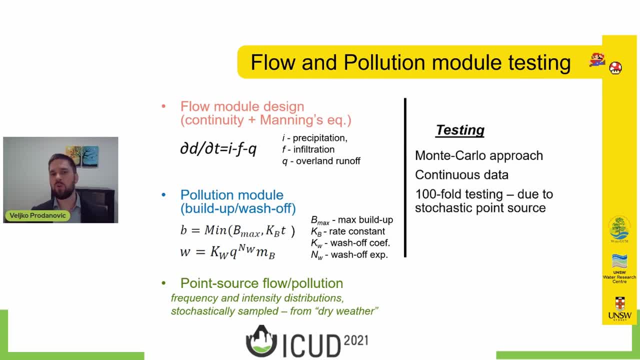 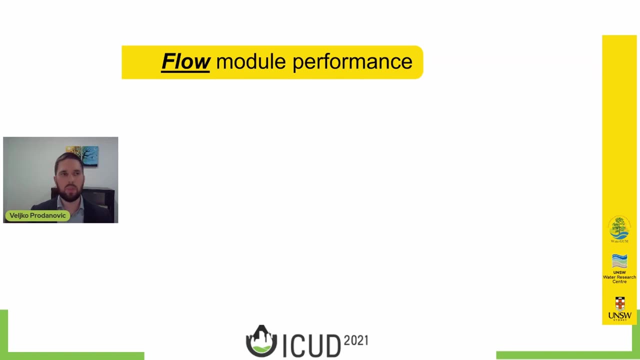 frequency and intensity distributions And the models were tested using Monte Carlo approach. on the continuous data- very important And because it has stochasticity, we used hundred-fold testing with an optimal parameter set to assess that stochastic relationship. Okay, So I'm pretty sure you're keen to see. 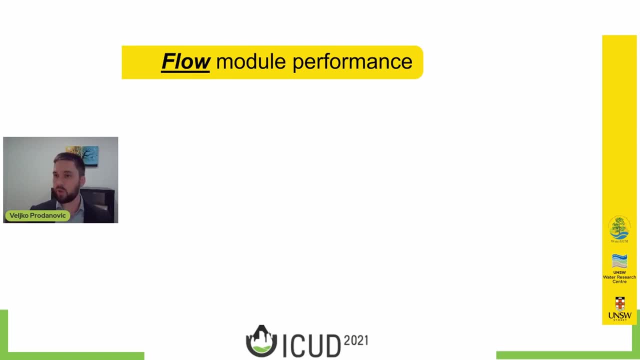 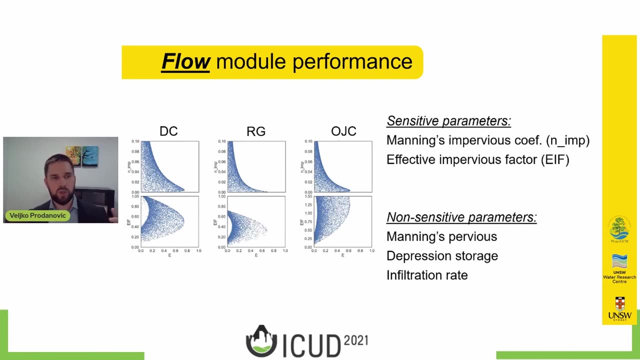 If this thing works. it seems simple, but does it work right? So we started from? we start from a flow model which started from seven different parameters, And sensitivity analysis showed only two parameters are sensitive. well, one kind of eh. 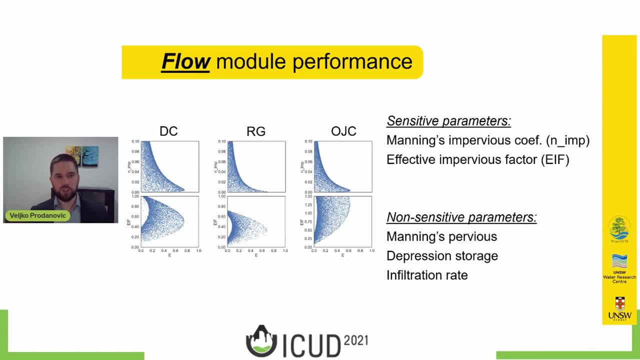 So we have a Manning's impervious coefficient, which is on the top row, which is sensitive, but below values of 0.01.. It's showing a low value of 0.01.. It's showing a low value of 0.01.. 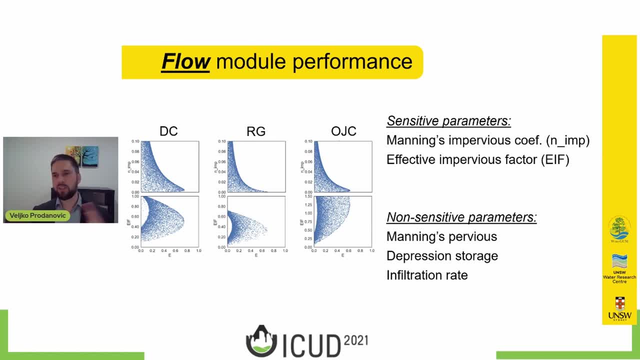 It shows less sensitivity across all different types of catchments and sizes. Another parameter was the effective impervious factor. Now, this is not a native SWMM parameter. This is an added parameter that accounts for percentage of directly connected impervious surfaces. 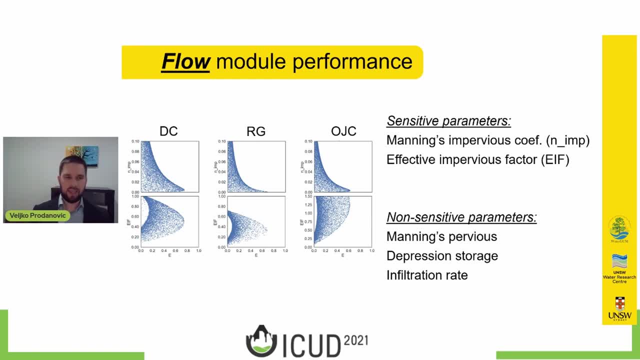 This parameter varied across different catchments due to the land uses and catchment sizes, So it's a true calibration parameter, while all other parameters of the SWMM were not sensitive. So practically we have Manning's coefficient of imperviousness, which is shows much less. 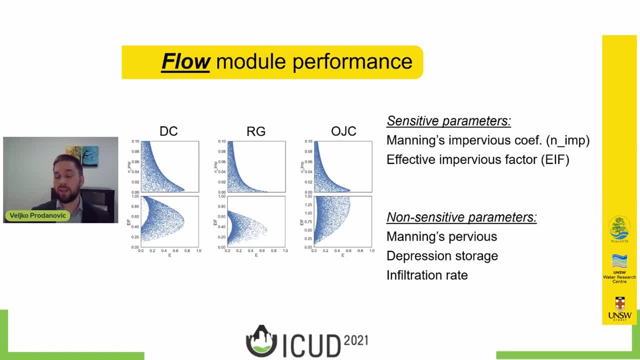 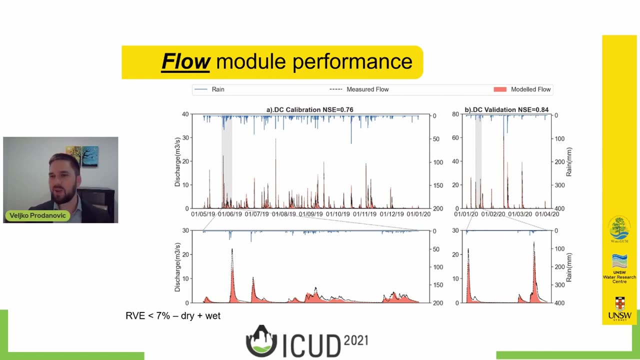 sensitivity below 0.01.. And we have only effective, impervious factor which can be calibrated. So that's great: One parameter for calibration. but how does it work? Well, we like it, I don't know. First time I saw it, I really loved it. 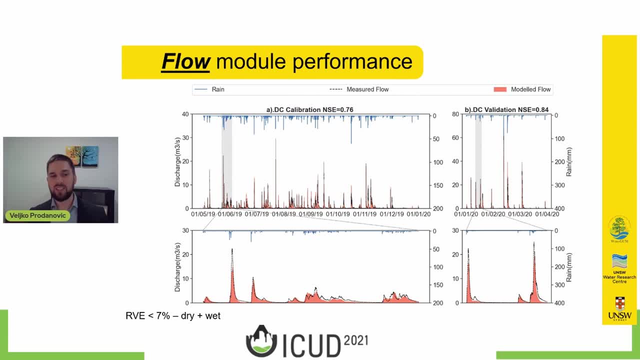 It shows really good fit across between measurements And I think it's a good fit. You can see that there's a lot of variance between the measurement and model values. with calibration on mind you continuous eight months' data of 0.76 of Nash-Dapflip efficiency. 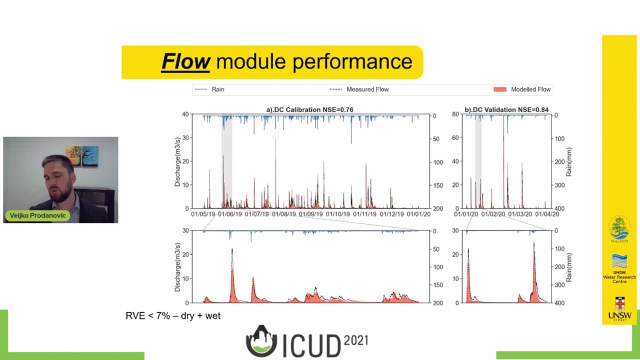 and validation showed even better results with three months of continuous data. So there are some extractions at the bottom of some of the events. You can see them better. So we have only 7% difference in relative volume error between the measured and model. 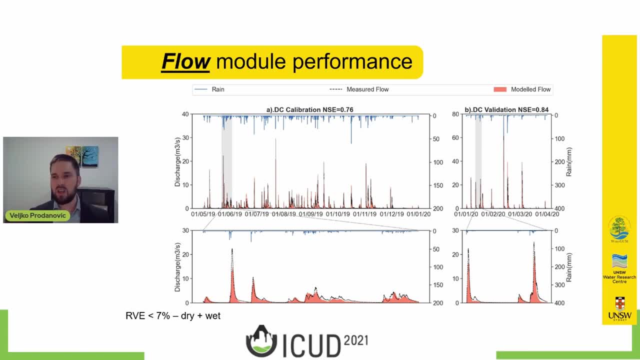 data, which is great, accounts for dry weather as well. So even with these simplifications, we achieved pretty good fit and pretty robust model, especially for flow, and basically has only one calibration parameter which, again for well-known catchments, it can be even estimated. So far, so good, right. 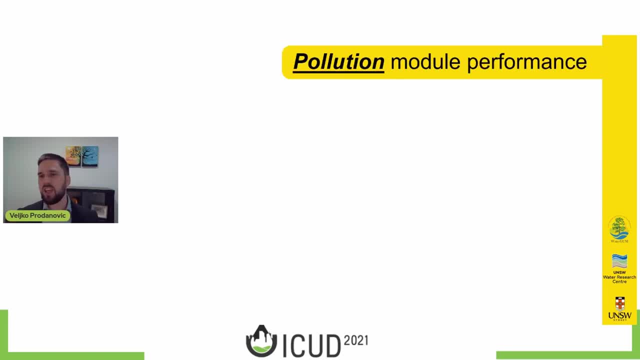 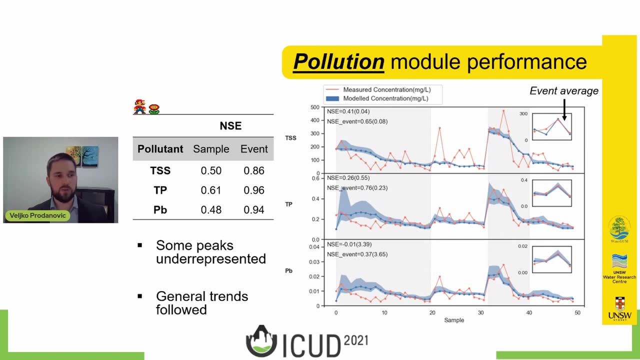 Let's now look at the tricky one. Let's look at the pollution. So the pollution module was somewhat more variable as expected. So we have total spent solids, phosphorus and lead- which still show a pretty good fit between the model and measured data, which is probably likely. 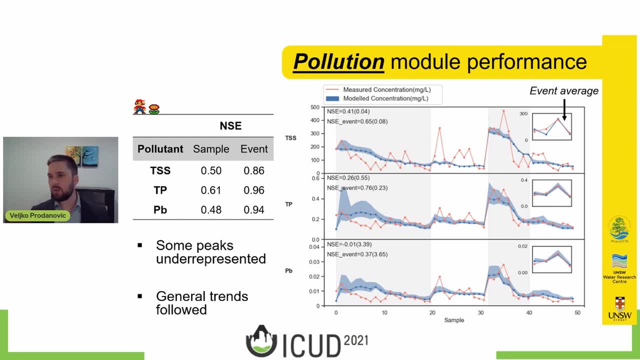 due to the correlation between the flow and these pollutants. So some peaks are still underestimated and this could be because these peaks might have been produced by the dry weather flow or the activities in the catchment which have been noticed when we were sampling. 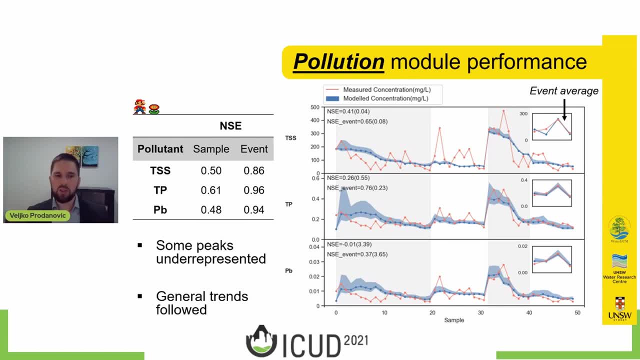 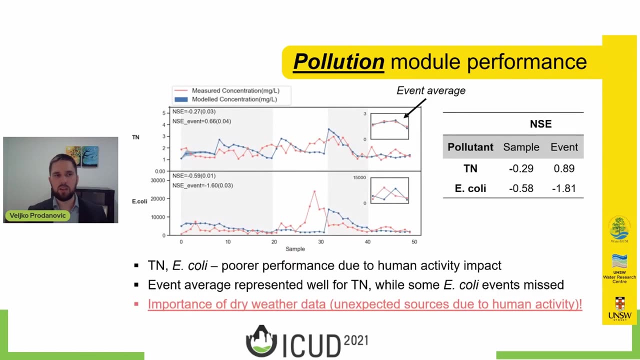 So our stochastic point source model was also a daily resolution, so we could not cover these intra-event periods. However, the averages- event averages- are pretty good and show a good fit, suggesting that aggregate pollution generation is well represented. Now the total nitrogen and E coli are somewhat poor performance. The trends are not followed. 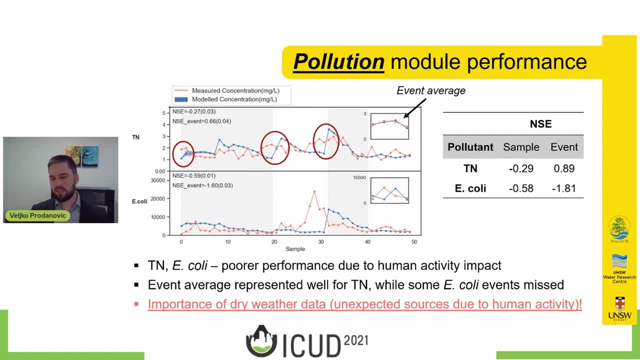 as well, especially at the beginning and ends of the events, where the contribution of the dry weather is the most significant. However, when we look at the event averages, again, nitrogen has a pretty good fit. So overall, we can still model the average daily concentrations and. 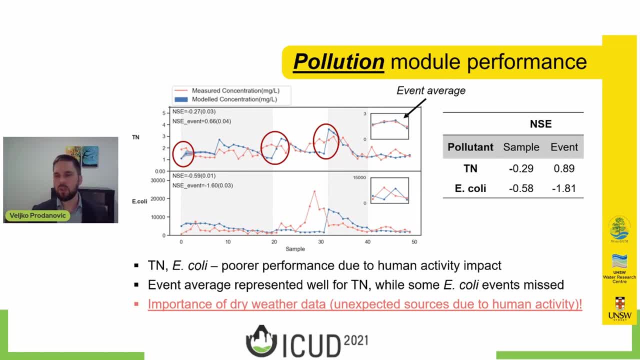 loads of nitrogen in our catchments. Again, because our dry weather generators- stochastic generator- did not have sub-daily values, those peaks could not be matched. So we can see that we have a pretty good model here, if I may say so, But how do we apply it for the future planning? 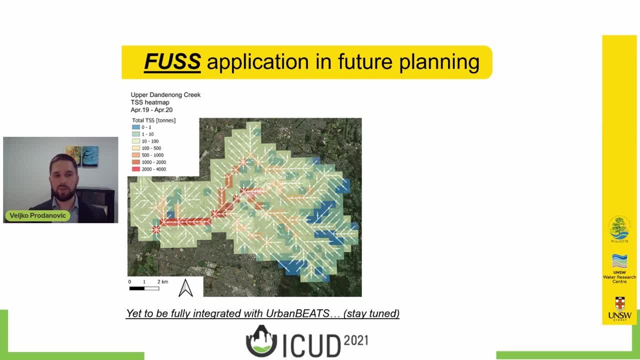 Well, one of the applications is to create heat maps like this, so we can see the distributions and patterns in our catchments, where the pollution flows and how it's going to flow. When we compare these to the future scenarios, we can see the differences. 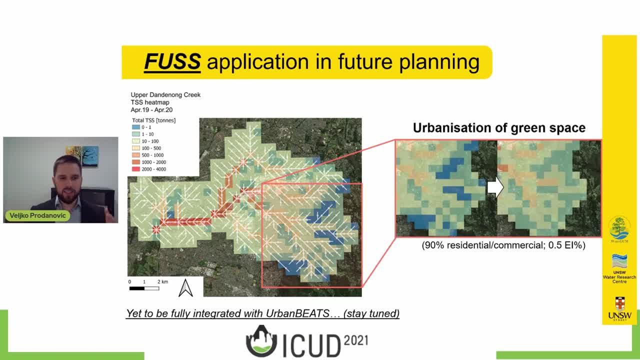 So let's play the devil's advocate for a second and let's urbanize our beautiful Dandenong forest and let's see what happens. So if we put 90% residential and we pave over 50% of the areas, we can see the definite changes in the TSS loads across the catchment and also 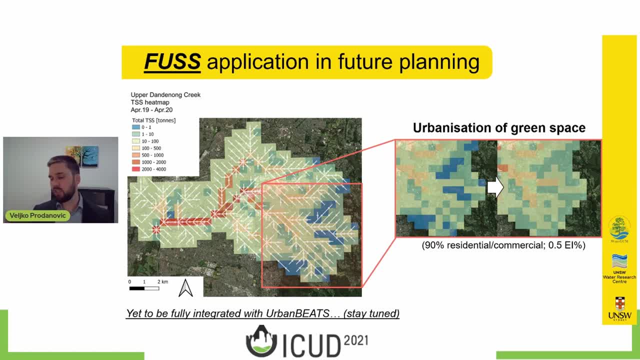 how it propagates. In a similar way, we can change the industrial land use and we can change all types of land uses and we can play around with population increase and stuff like that. So these scenarios offer us flexibility to interpret the model in different ways and to play around with the model Additionally. 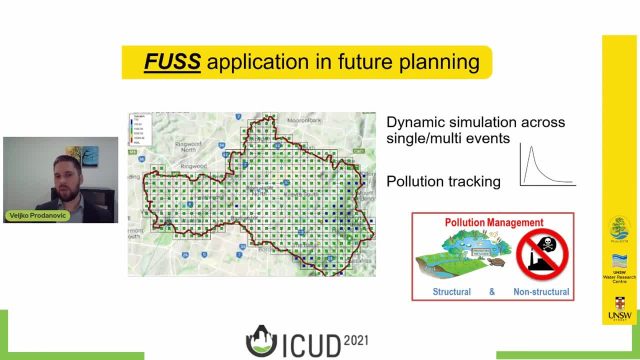 we can track the flows and pollution dynamically through the simulation because of the really fine time step of the model, which is only six minutes. So these pollution tracking will allow us to put pollution management strategies in place at the right spots at the right time. 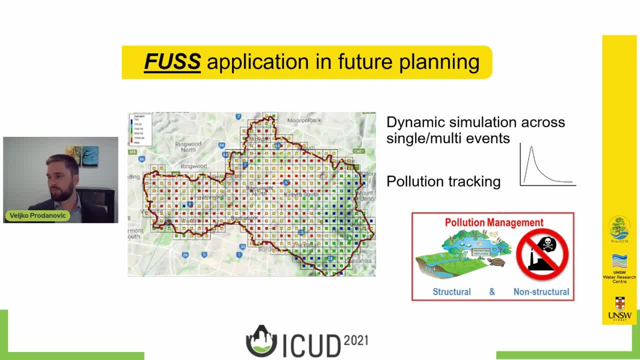 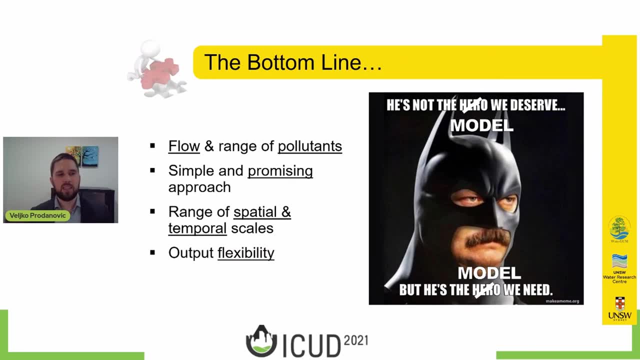 be them structural or non-structural, it doesn't matter. So the bottom line is: the flow and the range of pollutants simulated in this model have been pretty well estimated, and the model is still simple and has a pretty promising approach, considering the low input. 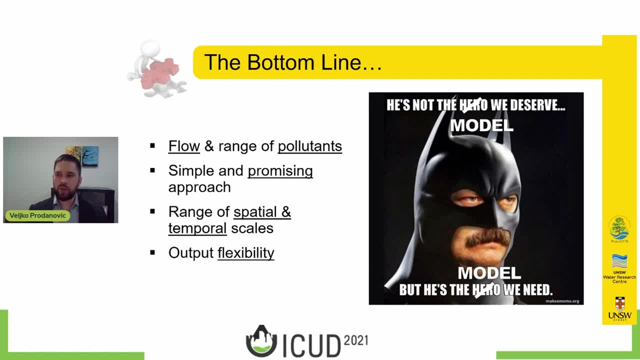 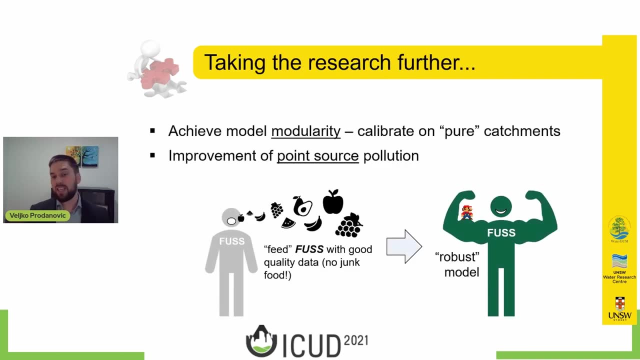 data requirements Due to the range of spatial and temporal scales and the output flexibility, as well, of the model. this might be the model that we need. We might not deserve it. we need it. So a couple of things that we can do better in the future is, if we want to achieve module modularity, 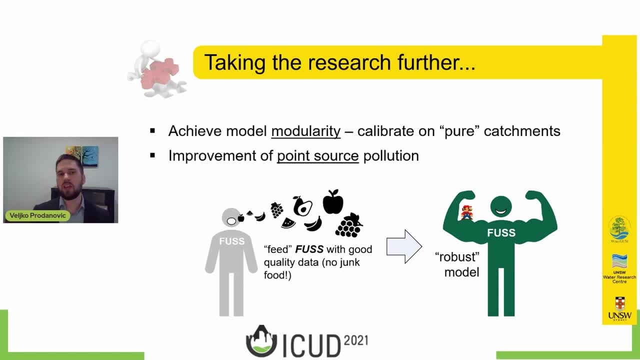 so we can apply this model without calibration on every specific catchment, especially for pollutants. we need to calibrate and create data sets for fewer catchments for every land use we can find, So this is something that we'll be looking at into future. 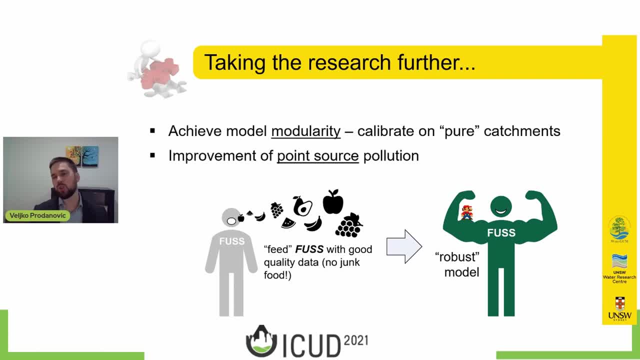 Also creating a model that's more flexible, trying to look deeper into these point- source pollution, trying to get subdaily values, trying to predict these peaks as they occur. So, in total, we're trying to feed the model, and with a good quality data. 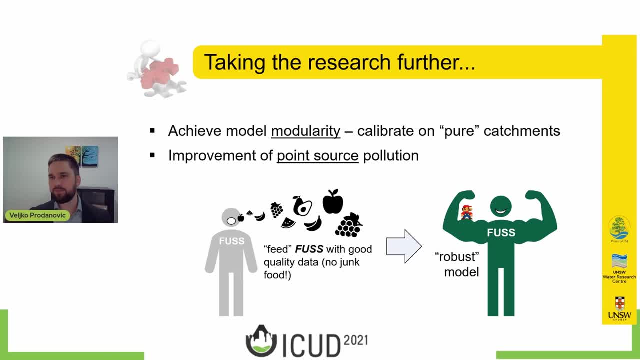 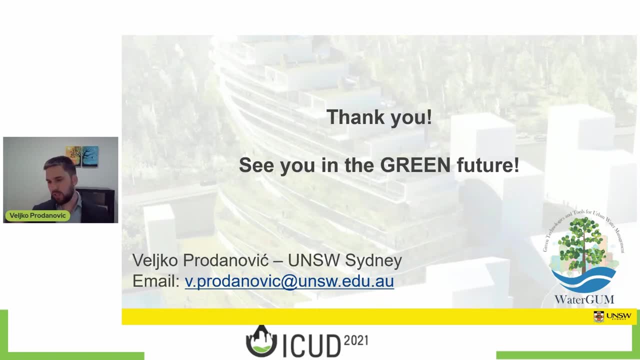 with a high, nice quality data so we can create a robust model that can be easily applied without pre-calibration. I'd just like to thank you all for attending this session, and all my co-authors on this work and all the people who invested a lot of time in this work. 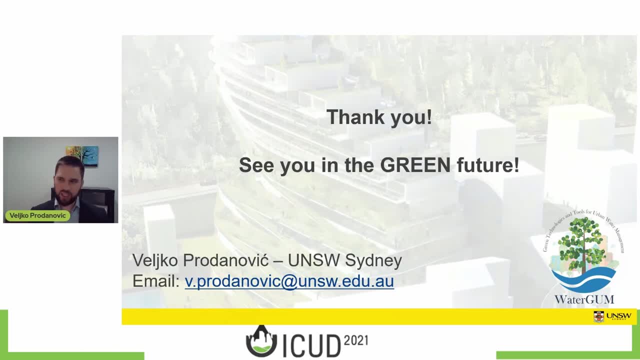 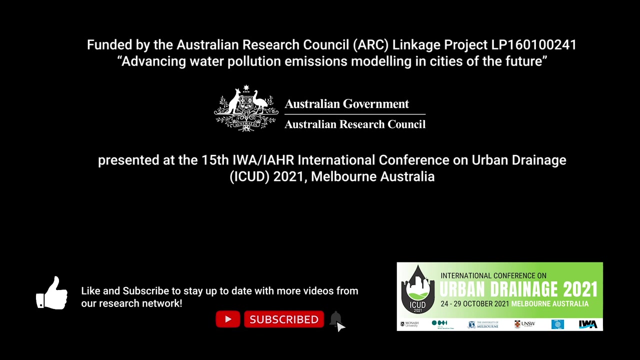 and I'm hoping that we'll all work together towards this nice, bright, green future, and also trying to inform those guys next week. if someone has a contact with them, please let them know. we're doing something good here, all of us. so thank you so much you.